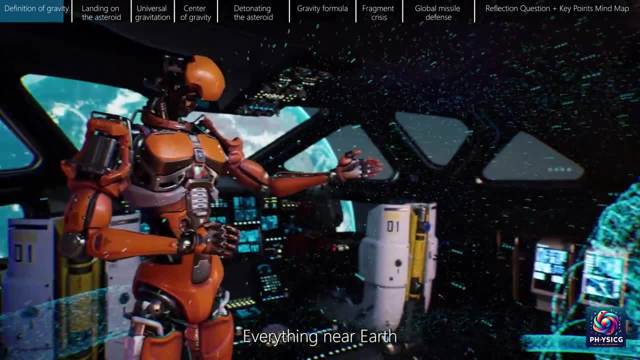 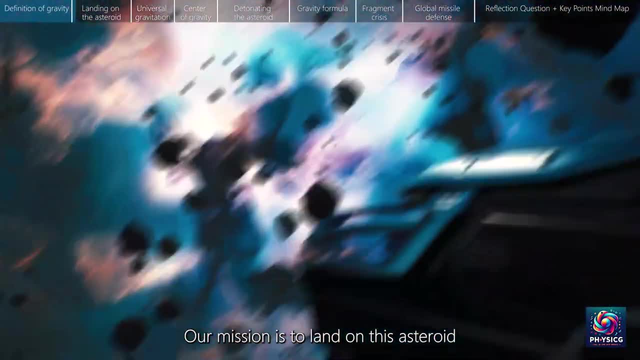 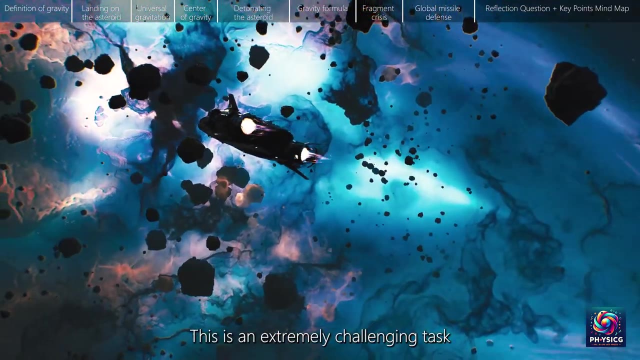 is called gravity. Everything near Earth, including our spaceship, is affected by gravity. Our mission is to land on this asteroid and use a nuclear bomb to destroy it, preventing its threat to Earth. This is an extremely challenging task. Our hopes rest on this. 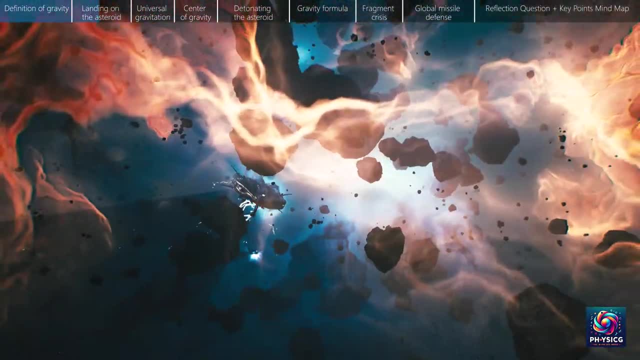 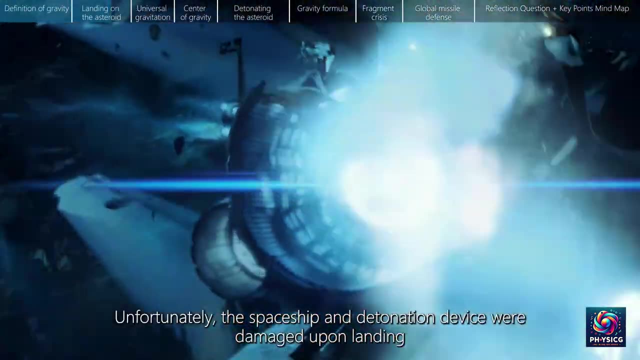 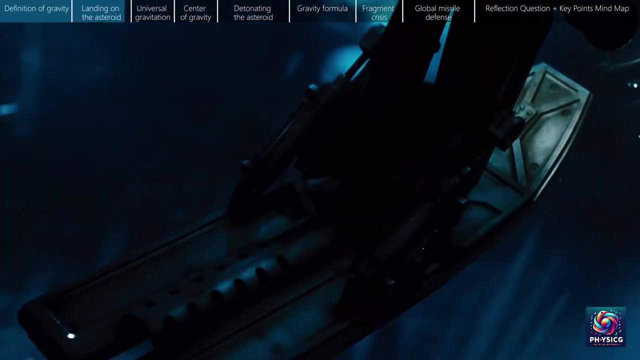 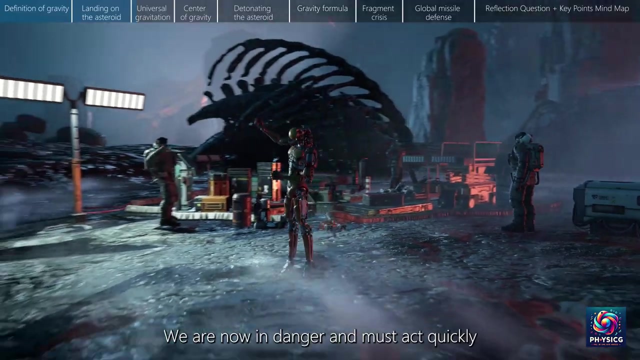 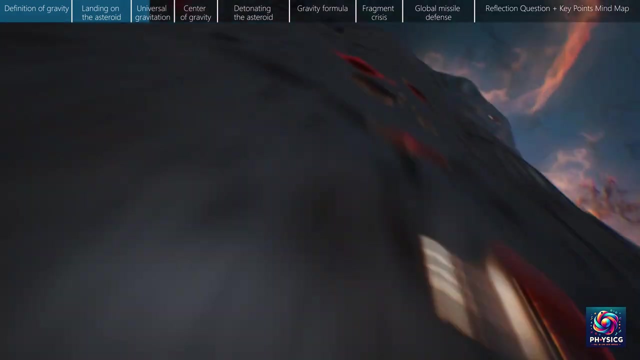 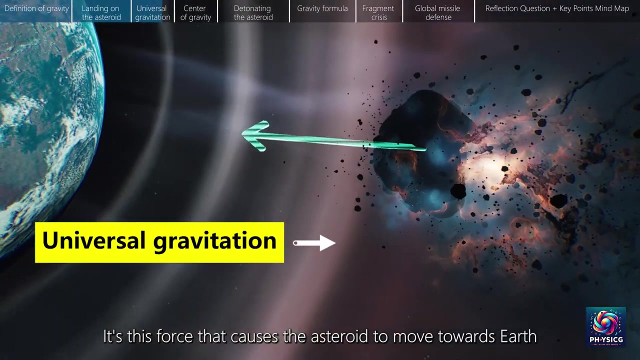 Unfortunately, the spaceship and detonation device were damaged upon landing. We are now in danger and must act quickly. The asteroid threatens Earth due to the force of gravity. Gravity is the force of attraction between all objects in the universe. It's this force that causes the asteroid to move towards Earth. 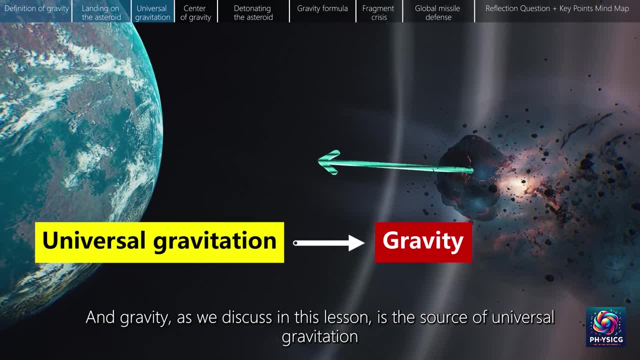 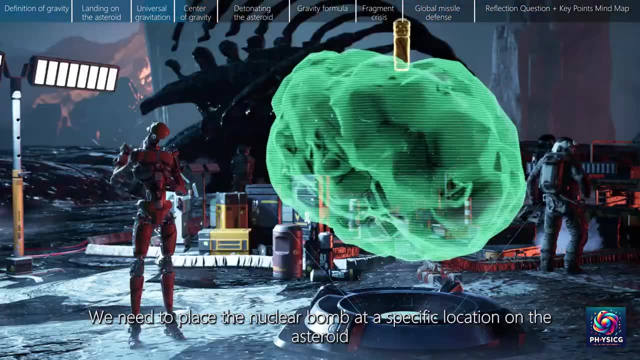 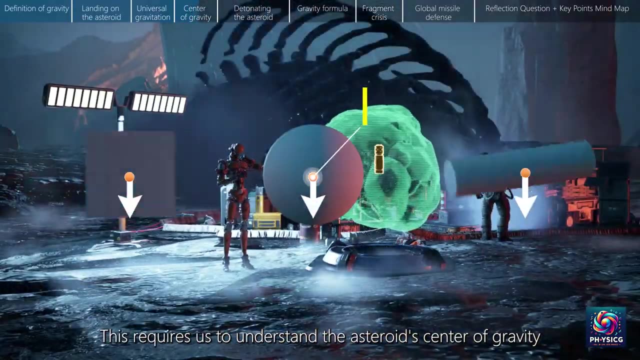 And gravity, as we discuss in this lesson, is the source of universal gravitation. We need to place the nuclear bomb at a specific location on the asteroid. This requires us to understand the asteroid's center of gravity. The center of gravity is the balance point of an object's mass distribution. 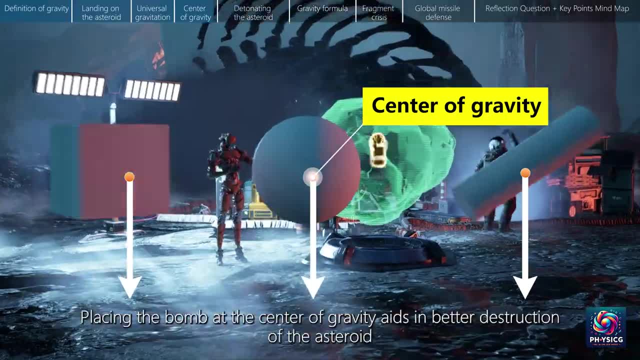 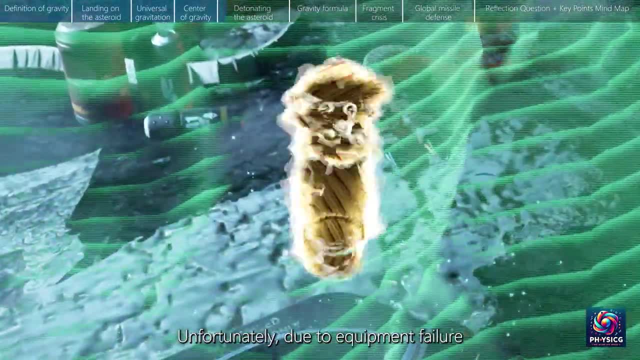 determining how it rotates and stabilizes. Placing the bomb at the center of gravity aids in better destruction of the asteroid. Unfortunately, due to equipment failure, we need a team member to stay behind and manually detonate the bomb. The others will evacuate. 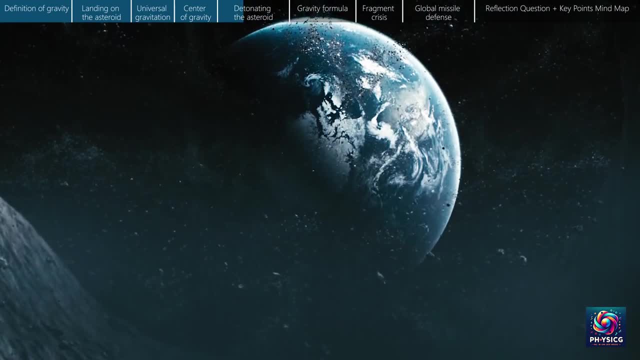 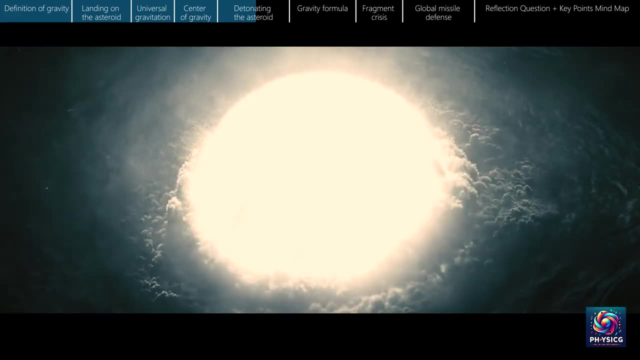 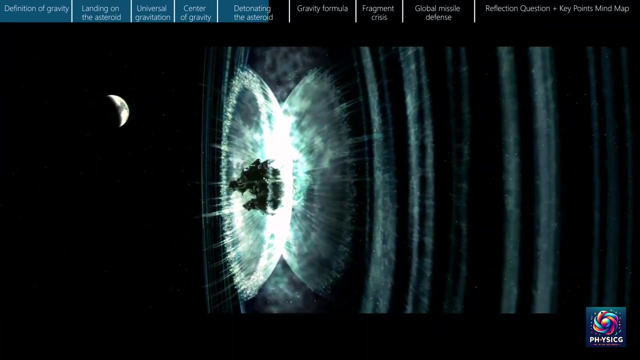 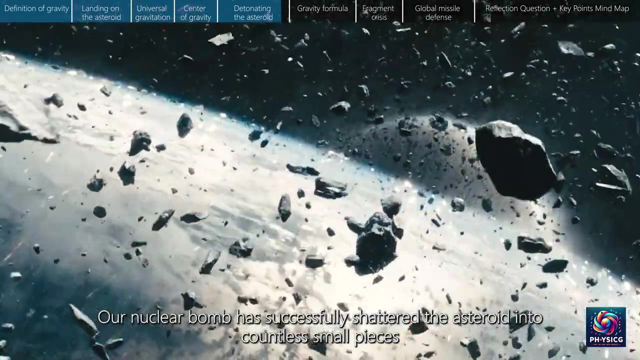 Thank you for watching. Please subscribe to our channel. We will be happy to help you. See you soon. альные 영상에 tribute reviews. Our nuclear bomb has successfully shattered the asteroid into countless small pieces, But now we face a new challenge. 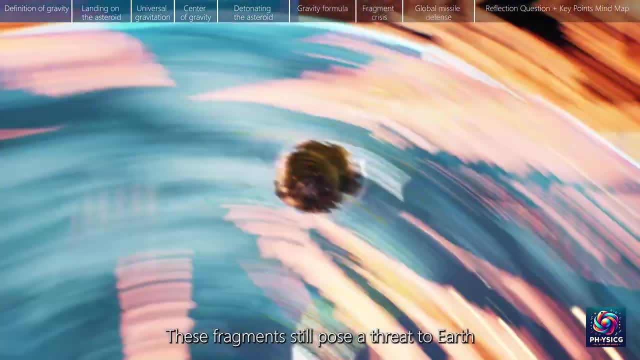 These fragments still pose a threat to Earth- Земля. To determine the fall locations of each of these fragments, we need to mine ore andробzent. To determine the fall locations of each of these fragments, we need to mine ore androbzent. To determine the fall locations of each of these fragments, we need to mine ore androbzę. To determine the fall locations of each of these fragments, we need to mine ore androbzę. commission me, про테 pence, and wish you stick with us. I wish I can do it Now. see you tomorrow, PUNCE. Thanks for having mines in throttle. 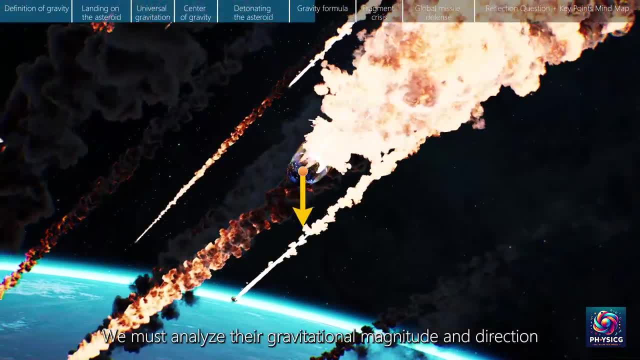 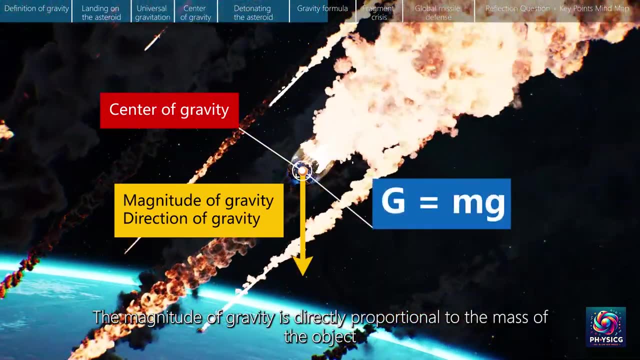 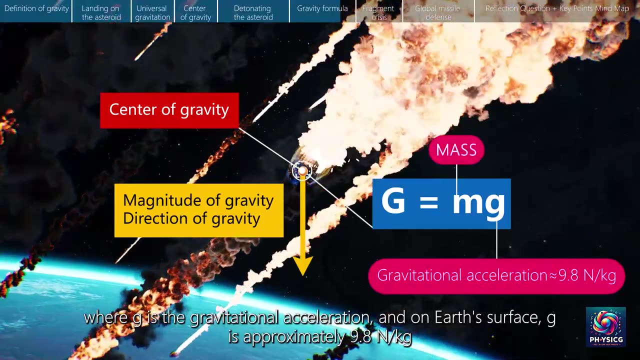 asteroid fragments, We must analyze their gravitational magnitude and direction. The magnitude of gravity is directly proportional to the mass of the object. It can be represented by the formula: G equals mg, where G is the gravitational acceleration and, on Earth's surface, G is approximately 9.8 n slash kg. It is 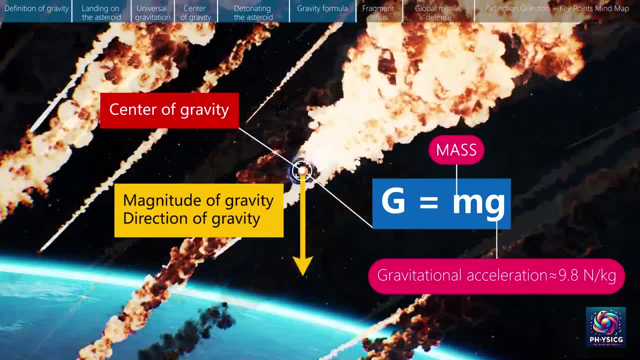 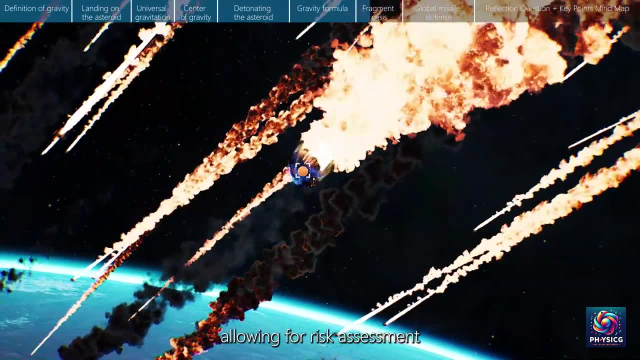 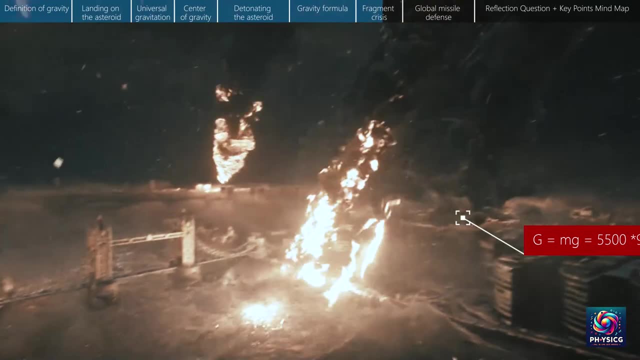 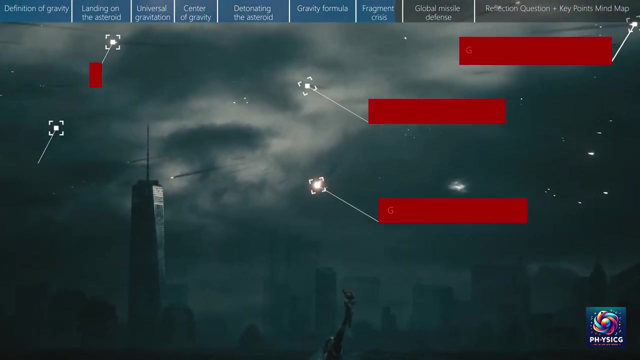 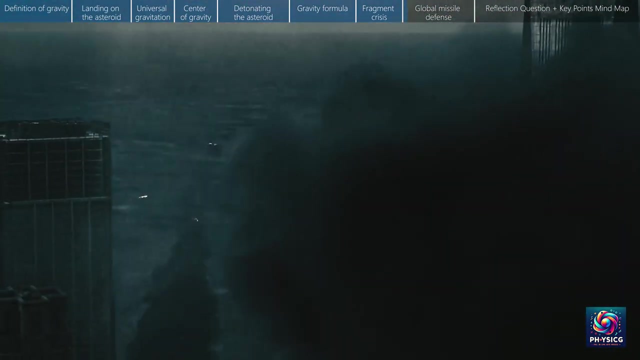 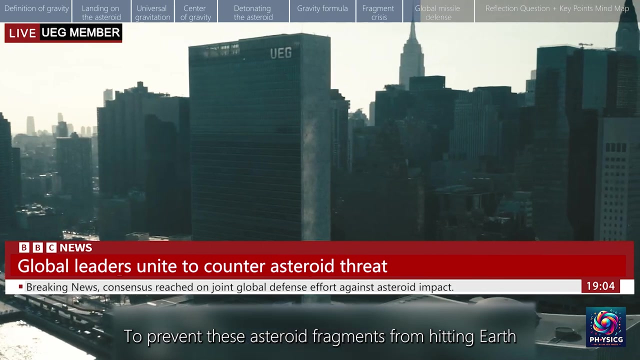 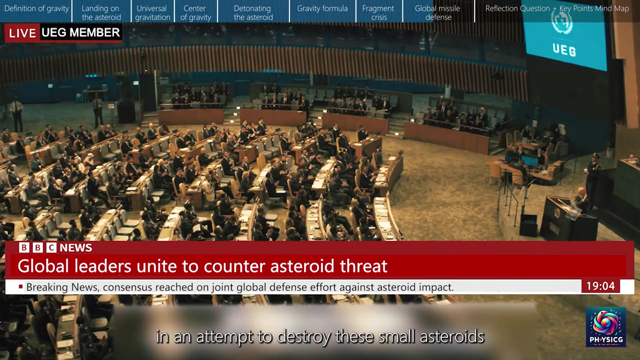 because the direction of gravity is always vertically downwards that we can accurately predict the falling locations of the asteroid fragments, allowing for risk assessment. To prevent these asteroid fragments from hitting earth, countries around the world have decided to unite to launch all available anti missile missiles in an attempt to destroy these small asteroids. 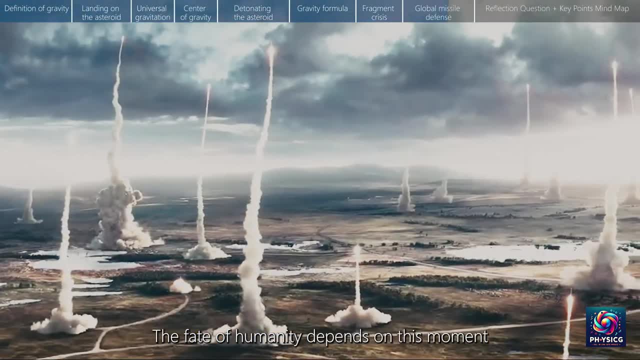 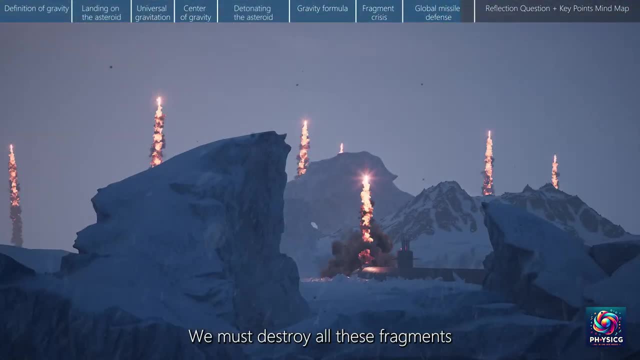 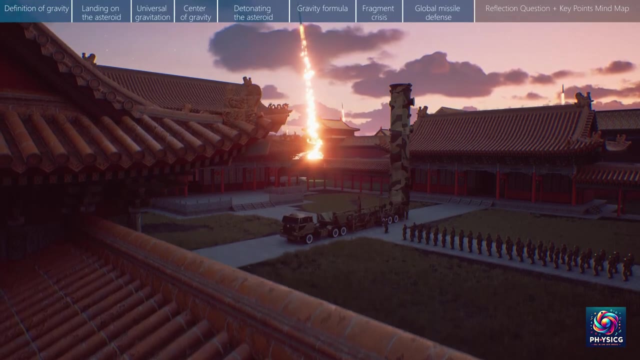 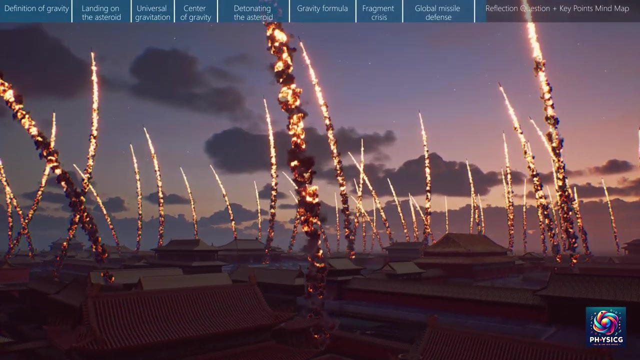 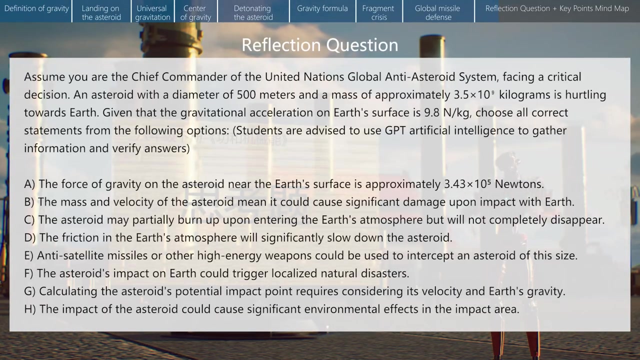 This is a true global effort. The fate of humanity depends on this moment. We must destroy all these fragments before they fall completely against the earth. fall to Earth. Students, this is a test for you. Assume you are the Chief Commander of the United Nations Global Anti-Asteroid System. 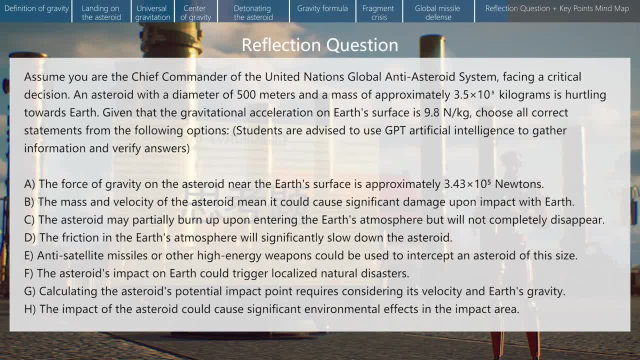 facing a critical decision. An asteroid with a diameter of 500 meters and a mass of approximately 3.5×10 kilograms is hurtling towards Earth. Given that the gravitational acceleration on Earth's surface is 9.8 n slash kg, choose all correct statements from the following options. 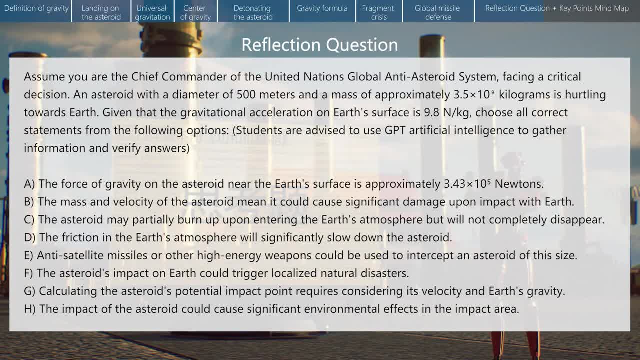 Students are advised to use GPT- artificial intelligence- to gather information and verify answers. A- The force of gravity on the asteroid near the Earth's surface is approximately 3.43×10 Newtons. B- The mass and velocity of the asteroid mean it could cause significant damage upon impact. 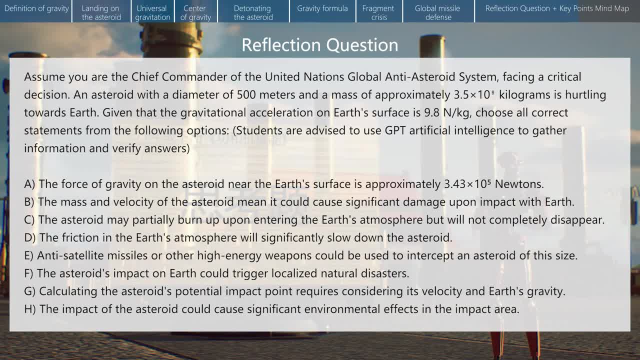 with Earth. C- The asteroid may partially burn up upon entering the Earth's atmosphere, but will not completely disappear. D- The friction in the Earth's atmosphere will significantly slow down the asteroid. E- Anti-satellite missiles or other high-energy weapons could be used to intercept an asteroid.